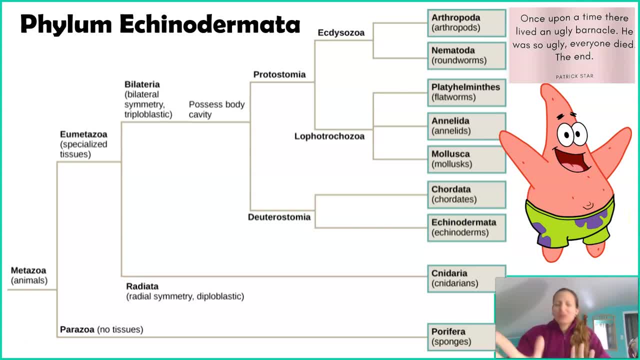 Welcome to phylum echinodermata, And I'm just going to pause right there. I have Patrick Star on here, so you can probably get a guess as to which group of organisms this includes. But if we just pause and look at the word echinodermata, we can actually kind of deduce what organisms are. 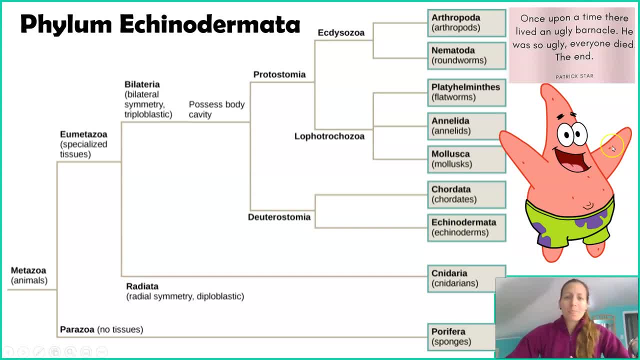 in here just based on the name of the phylum, So you might be more familiar with derm. Remember derm is referring to an outer covering or a skin, And maybe you're not as familiar with ekin or ekinome. Maybe you've heard of the animal echidna, which is a spiky animal Ekinome refers to. 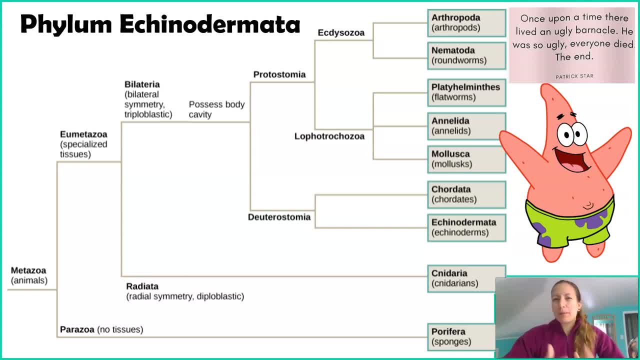 spikiness. Sometimes people will say bumpy, but it means spiky or spiny, So this is referring to organisms with spiny skin. Now, you might not think of a sea star as having spiny skin, but if you actually look closely at it and feel it, it definitely does. But this also includes 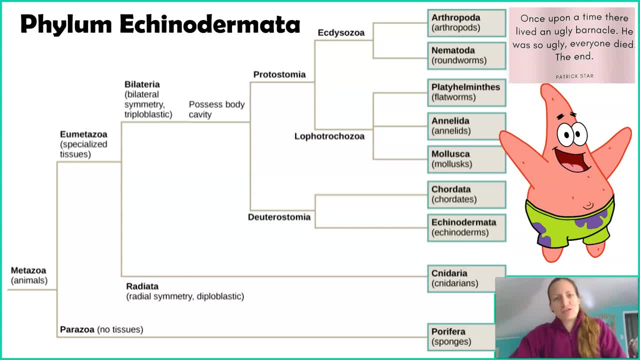 our sea urchins. So taking a look at the phylogenetic tree of our animals, So we are in the eumetazoa, so pretty much our true tissues. We are in bilateria, or the bilateral organisms, And you might be pausing and be like: well, sea stars aren't bilateral, but we'll touch on that. 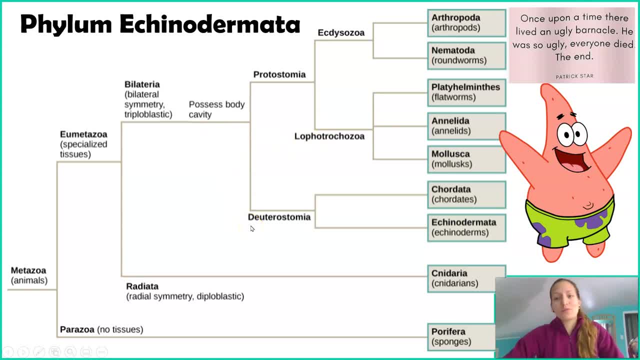 soon, And now we're going into our deuterostomes. So in our deuterostomes we have two groups of organisms: Echinodermata, which we'll talk about in this video, And then in the next video I have, we'll talk about Chordata, which is what we're found in So 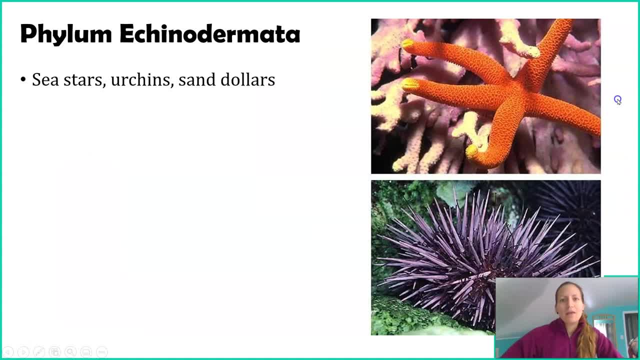 let's go ahead and dive in to learn more about these guys. So, as I mentioned in the previous slide, this includes things like sea stars, sea urchins, like you see here, and sand dollars. You might be familiar with sand dollars because you especially if you go to a beach house or 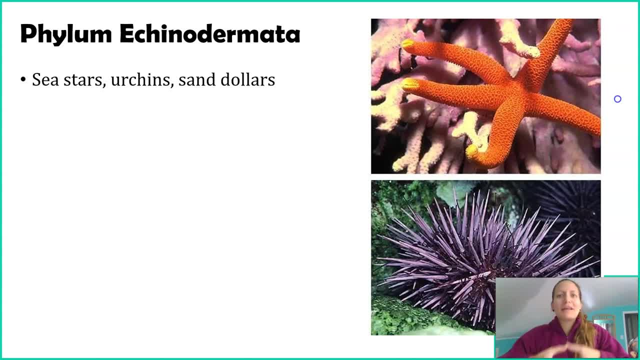 somewhere that's coastal themed, there's probably those dried sand dollars. They're probably those dried sand dollars. They're probably those dried sand dollars. They're kind of white little circles. They usually have little designs in the middle of them. That's the skeleton of that Echinoderm. They use the word skeleton kind of lightly. 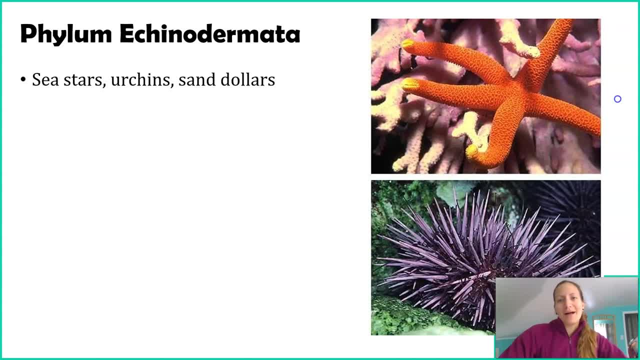 but yeah, it's just, it's a dead animal that's on someone's you know mantle or on their on their kitchen table. So all of those organisms in their live form have this spiny skin, And in the bottom right corner here that's an example of a sea urchin. Tons of different. 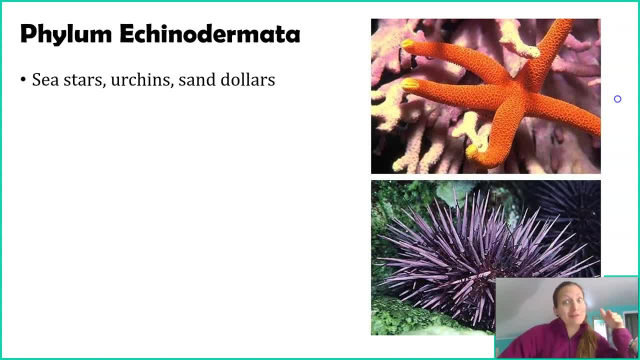 species out there And that's like definitely some spiny skin. So let's talk about this symmetry Now. in the phylogenetic tree, this group is combined with all other organisms in bilateral symmetry. But if you look at these, these guys are clearly radially symmetrical And this is 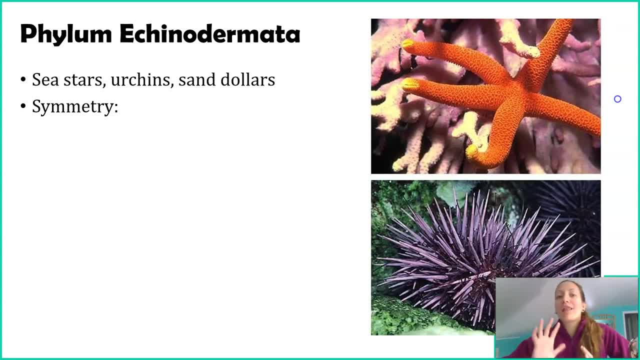 where this group gets kind of weird. So as long as you're looking at these organisms, you're going to see that they're bilateral. They're not just larvae, So not the adult form As larvae, they're bilateral. They kind of share those early embryonic stages with other organisms with bilateral 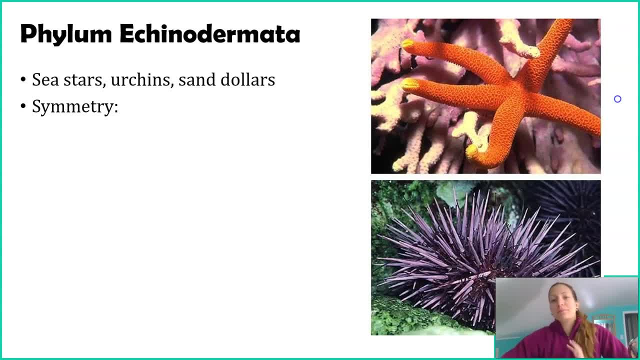 symmetry, So as larvae they're bilateral, And because they're sharing that with ancestors that are also bilateral, we just keep them organized with bilateral. However, very clearly, as you see in these two pictures of adult Echinoderms, the adults have radial symmetry, And so they're kind of 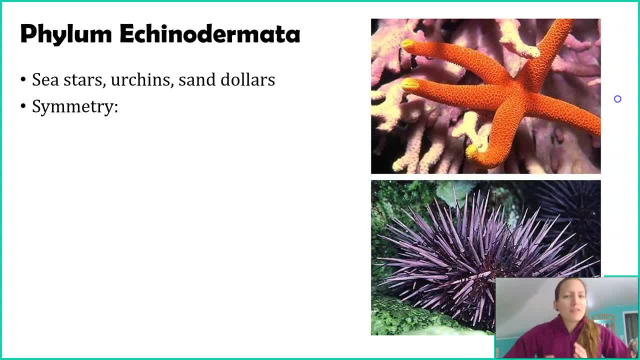 not in that radial symmetry. So you could argue they have both. It just depends on which part of the life cycle we're talking about. As far as Diplo or Triploblast, this is going to be a triploblast, So they have those three germ layers And the way those germ layers are arranged is, as a 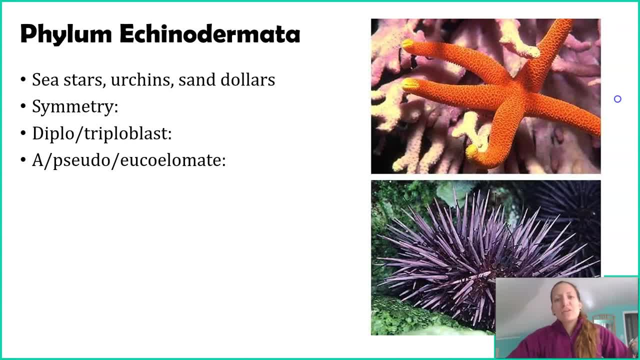 eusealomate. So they have a true coelom, That mesoderm is lining all parts of that body cavity And this is. these two characteristics are what we've been seeing for a lot of our animal phyla. They do have complete digestion. Now, if you're looking at them you're like, do they? 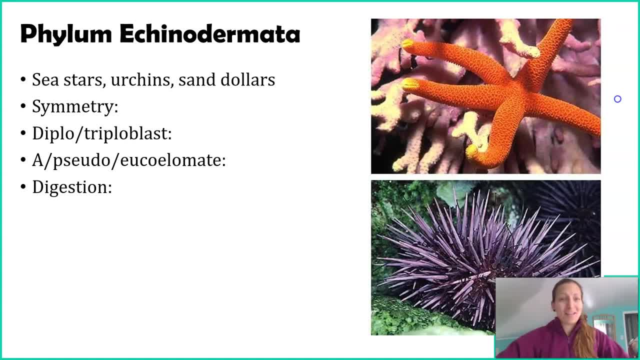 I don't see anything. I see no mouth, I see no anus. Like, do they have any digestion? They definitely do. We'll explore it more on the next page, though- But they do have complete digestion, meaning they have separate opening, one for the mouth, one for the anus. And because 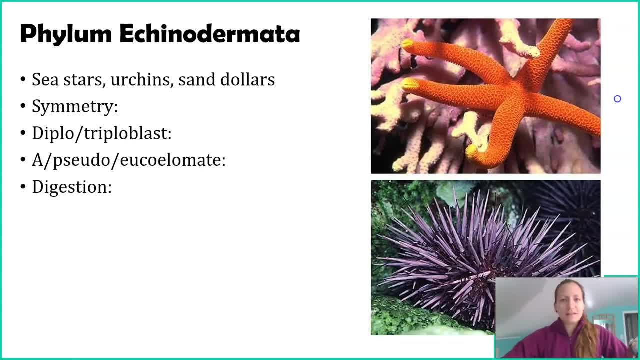 they have those two openings. that means we can designate them as either a protostome or a deuterostome. One of those openings had to form, first And of all, the animal phyla we've talked about. this is our first group that is a deuterostome, So remember, deutero means second. 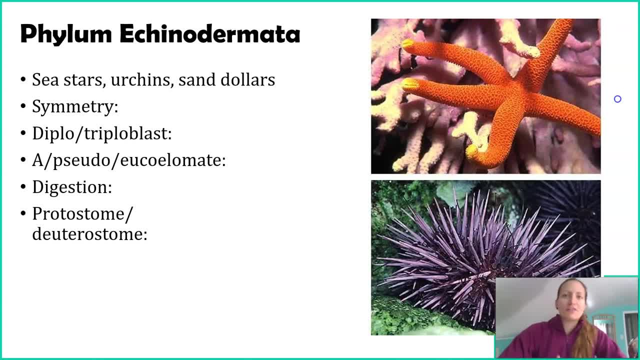 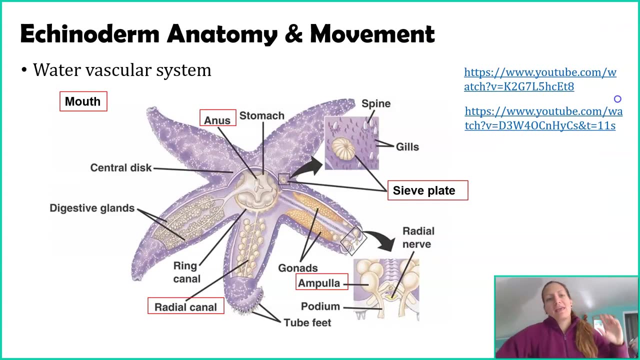 and stome, referring to mouth. So the mouth is forming second or the anus is forming first. Same thing. So these are kind of our basic characteristics of Echinodermata And let's explore something I think is cool about them And it's how they move. So this is looking at a sea star, but all Echinoderms move this way. 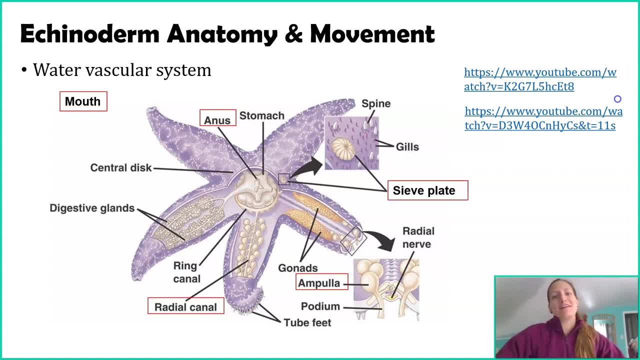 And they move through something called a water vascular system. Now I'm going to pause. Before we even talk about this system, let's talk about movement of other things Like humans. When we go to move, I would show you walking, but you're not going to be able to see that When you move. 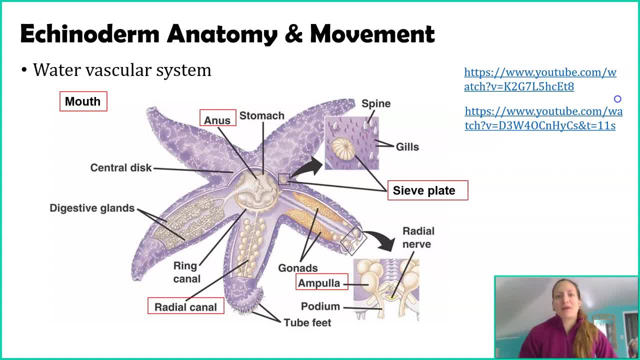 oh god, relaxing of your muscles. right, It's your muscles that help you move, As well as, obviously, your skeletal system is needed, your nervous system is needed, but for the most part, it's your muscles that are doing the work, And with a lot of organisms, it's the muscles doing the work. 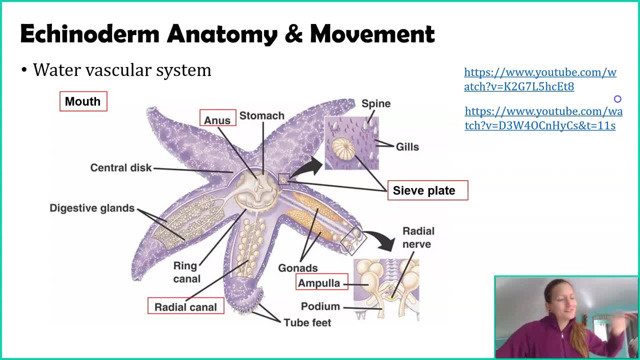 But Echinoderms are like: nah, we're going to do something different. They're like: let's use water. We're found in water, Let's just use water. So Echinoderms have a vascular system. Again, I keep using humans as an example, because you're probably 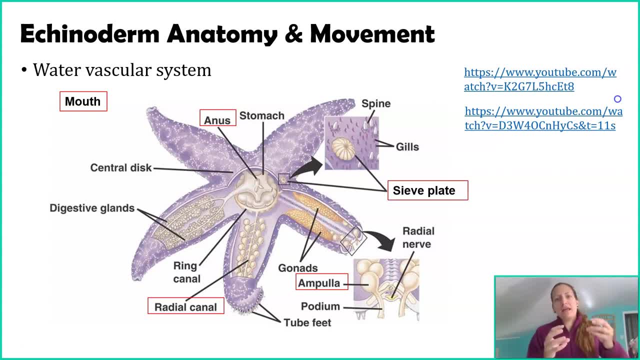 most familiar with humans. So vascular system is typically a series of tubes and canals and vessels that are moving stuff. In humans it moves blood, it moves oxygen, it moves nutrients, it moves wastes. In Echinoderms they have a series of tubes similar to our vascular system. 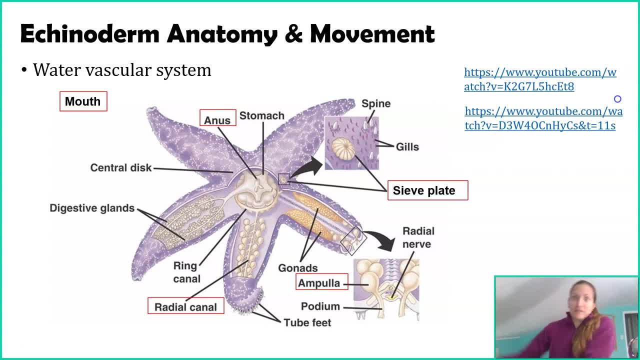 but it's water, And it's not just any water, It's the seawater, It's just water they're getting from their environment And they're using that to move, which is crazy. So let's talk about that. So I'm going to use this sea star as an example. 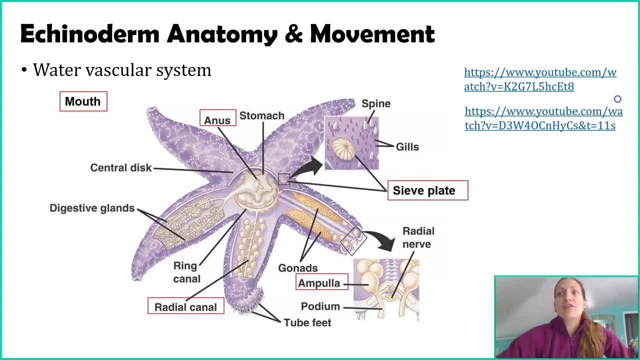 but again, this applies to sea urchins, sand dollars, sea cucumbers, all of the organisms found in Echinoderms. Now you'll notice, on this particular picture it has a lot of different words. I'm going to really just highlight the ones in red. Those are really the ones I care most about. 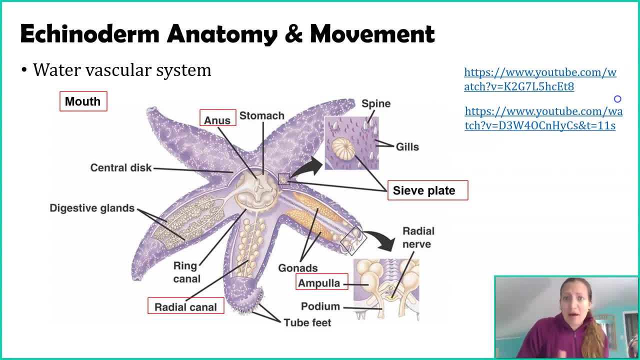 So first we will mention there is a separate mouth and anus on our sea stars and all of our Echinoderms And it's actually in the same general area on each of the different organisms. So the anus is actually right on top of the organism or the dorsal side, And it's usually 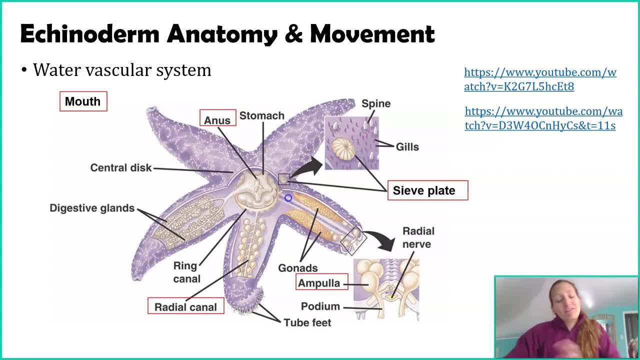 incredibly small. You likely, even if you had a dried specimen, you likely may have a hard time actually finding it. They poop kind of like how fish poop, where it's like a really skinny little thing, So you likely wouldn't even see it. but that's found on the top side, or the non-feeding. 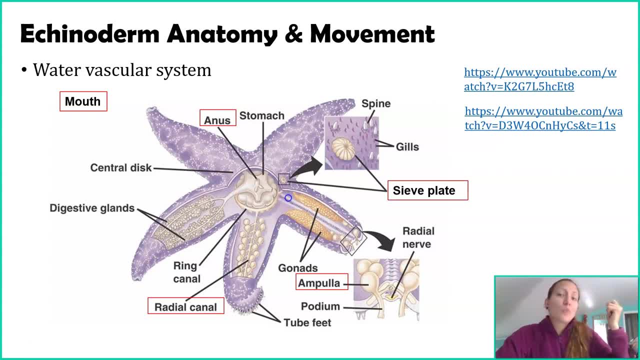 side of the organism. Remember, with radially symmetrical organisms you usually have a top and a bottom side, a feeding and non-feeding side, So the anus is on the top And then the mouth. it's labeled on here but it's not pointing to anything because that's found underneath. 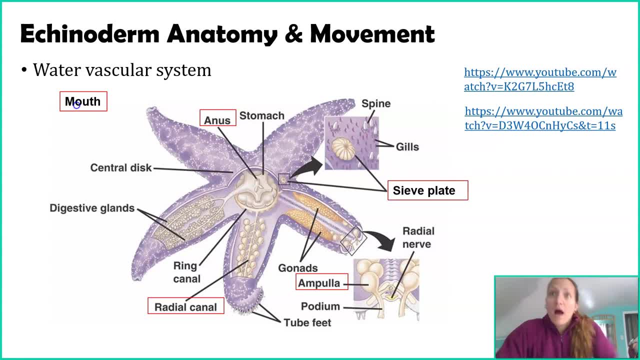 the sea star. So this is where a much larger opening is that you can definitely see on all of our different Echinoderms. And it's gnarly, And one of the videos I'll have you guys watch shows you up close and personal a sea urchin mouth just chomping away at some kelp. 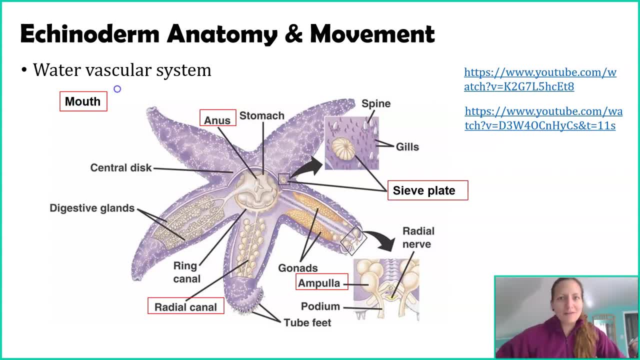 So that's where the mouth and anus is. Let's talk about this water vascular system, though. So the first thing that needs to happen is water needs to be taken in into the Echinoderm. But here's the thing: Like you could just have a hole that, just like it, sucks it in like a mouth, or 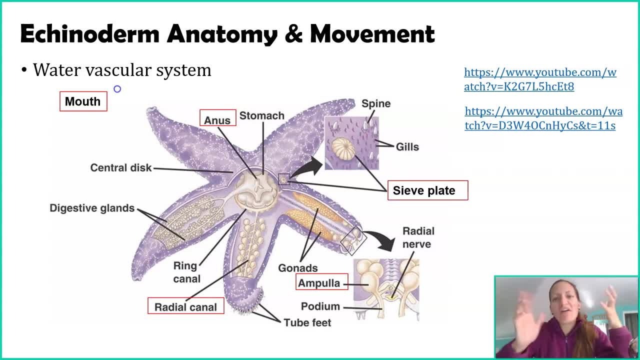 something. But you could have a hole that just like it sucks it in like a mouth or something. But there's stuff in the water And if you're sucking in this water to travel through pretty small vessels in your body, it's really important that there isn't stuff in your water. So, yes, 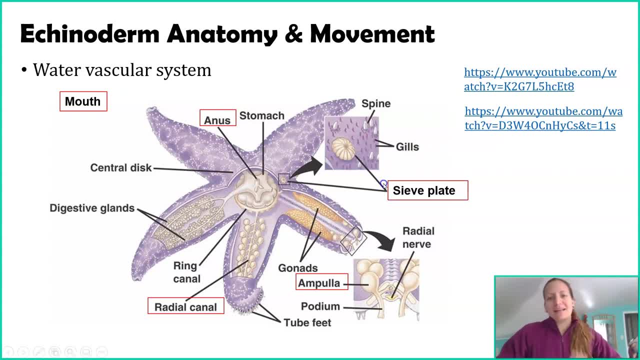 the sea star sucks in water but it goes through something called a sieve plate And if you know what a sieve is, maybe if you went to the beach as a kid you may have had like one of those little pans And you know what a sieve plate is. It's a little thing that you put in the water and 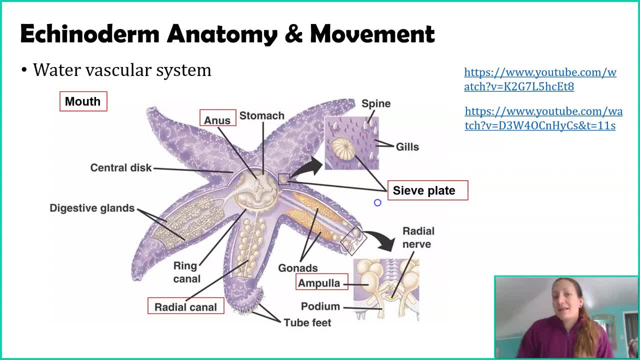 you like shake it and you're like: oh, there's cool shells that come out. That's a sieve, Like that's the official name of those tools. So a sieve plate does the same thing: It filters and sucks in water at the same time. And again, it's because you want clean water. 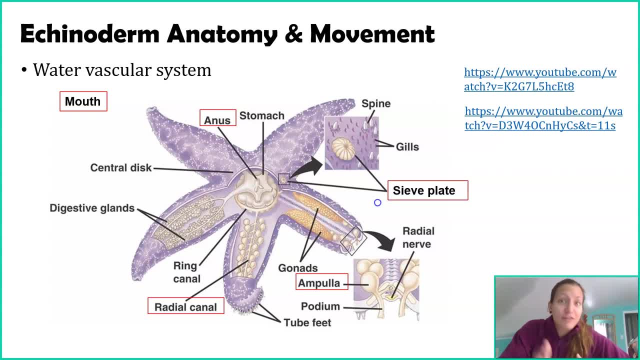 traveling through all your vessels. There is another name for this. I will use the term sieve plate. I'll keep using the word sieve plate, but you might hear it in one of the videos. You might see it on the internet. You might hear it on the internet. You might hear it on the internet. 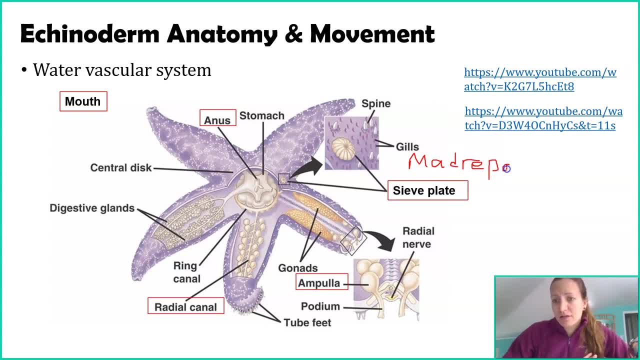 You might hear it on other diagrams: The madriporite. Again, I expect sieve plate. I'm going to use sieve plate But in case you see this word, you're like what are they talking about? The madriporite is another word for the same exact structure. So water gets sucked in. 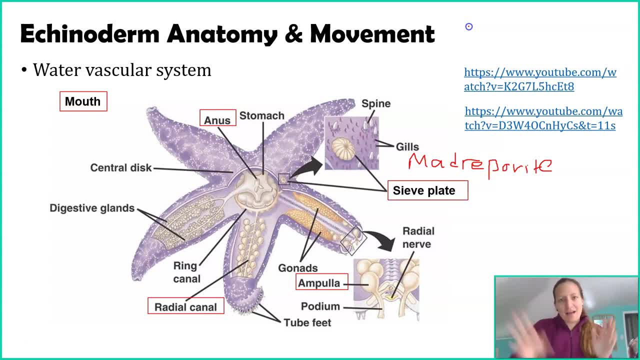 to the sieve plate. All the other stuff kind of just stays on the outside. Then this water travels through something called the radial canal. So the water comes in and it's going to start going down these radial canals. Think of radial because you know it's. 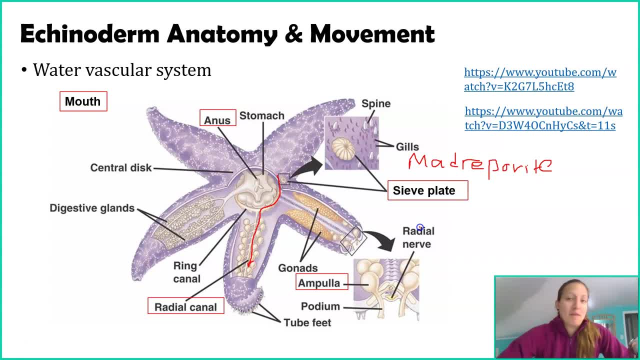 like I don't know, radial symmetry. Maybe that's where the name came from, I don't really know. In the case of a sea star, there's one radial canal going down every leg right The legs being used for movement. There's other sea stars that have 20 legs. 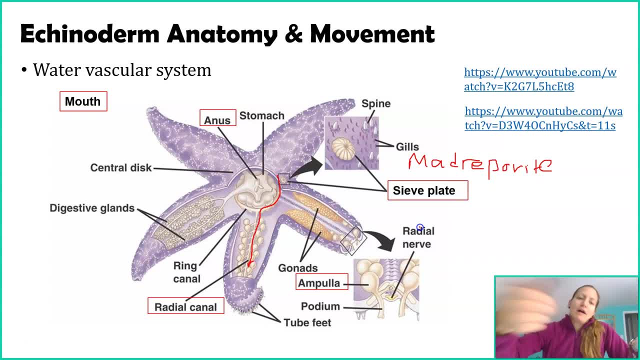 There'll be 20 radial canals. So radial canal goes down each arm. So water is coming in through that sieve plate And then it's going to start going down these radial canals. Think of radial because you know, water gets sucked in to the sieve plate. It's going towards each of these radial canals. 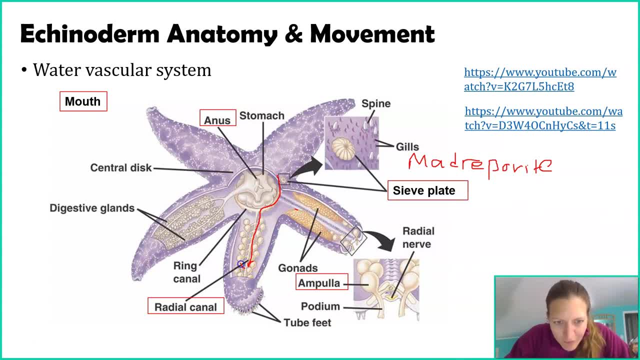 Then what happens is water fills these little tubes called the ampulla. So over here, this is a close-up of here's our radial canal coming down with water and they're going to fill up the ampulla. I'd like to think of ampulla as turkey basters, If you're familiar with a turkey baster. 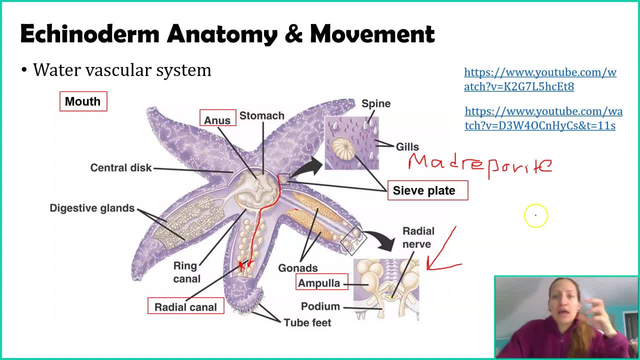 if I had one I'd show you That'll make enough turkey to have one. So it's a turkey baster, has like a big bulb at one end of it and then it's like kind of a long tube. You're supposed to use it to suck up turkey juices and then push that turkey juice. 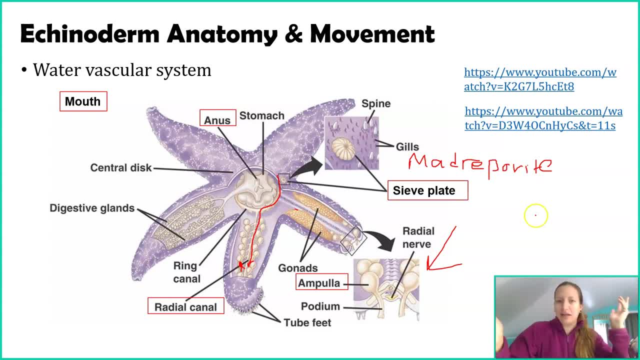 back out over on the turkey. Get a nice, beautiful, yummy. turkey Ampulla work nearly identically. Water comes down that radial canal, fills that ampulla. So the ampulla is now filled with water And there are still muscles involved. 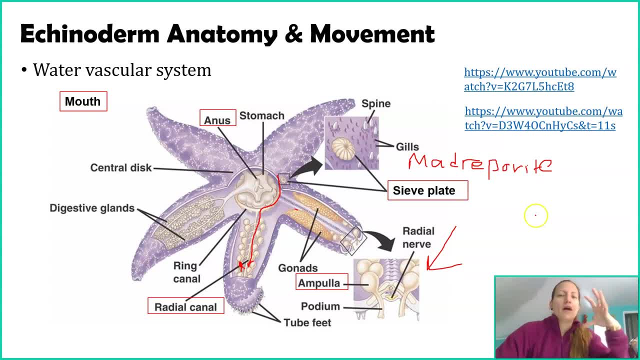 However, what the muscles do is they push the ampulla, They squeeze the ampulla so that the water comes out of them. Now, if you've ever used a pipette, like one of the plastic ones or a turkey baster, when you push out the liquid in them, it comes out with some force- Not a lot, but some. 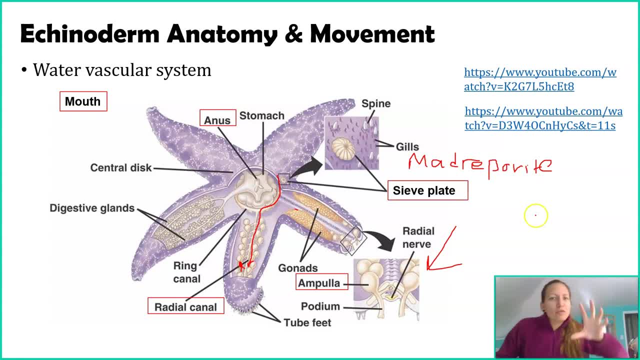 force, And so what's happening is, as the ampulla gets squeezed and water gets pushed out of them, causing it to move forward, Those muscles are moving it in such a way that that momentum, from squeezing out that liquid, is being used in a forward motion- I shouldn't even say forward. 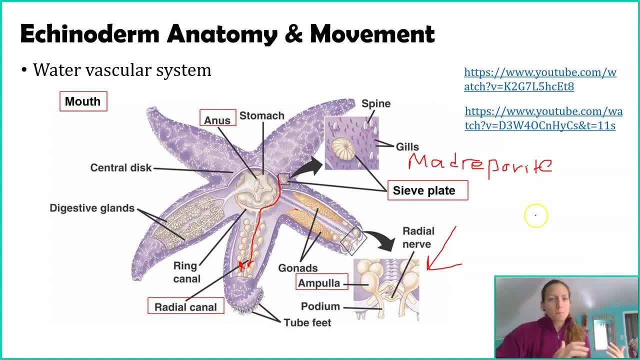 It could be any motion. The sea star can move in any direction, but it takes work. All right, We talked about one of the downsides of radial symmetry is that it takes work to move, to coordinate a particular direction, because there really is no forward or backward or 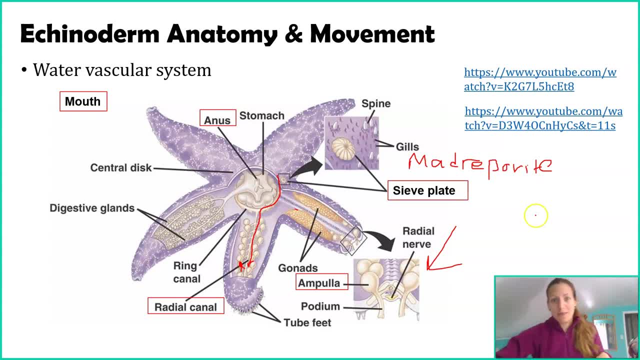 side to side, It's equal all the way around. Now there's hundreds, thousands of ampulla that these sea stars are coordinating in order to go in a single direction And because that coordination is a loss. that's why they move slowly. But it's cool because they can move. 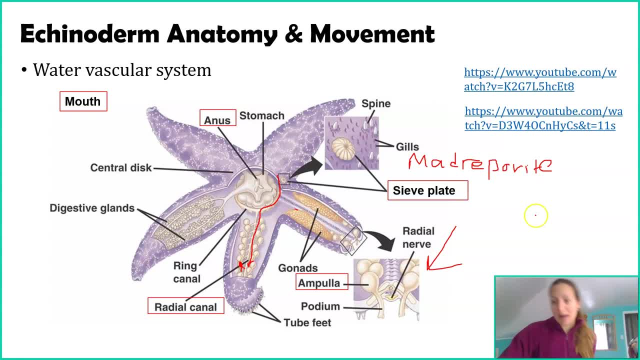 with equal ease in any direction. It's just configuring the direction of those ampullae. So, although I'm using the sea star as an example, again, this is happening in all of our echinoderms. They all use a water vascular system in order to move. They all have the anus and the mouth in